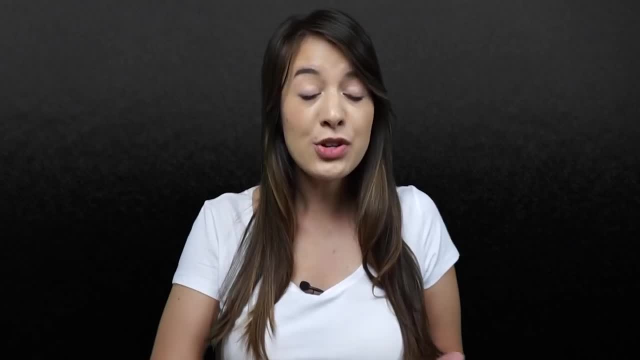 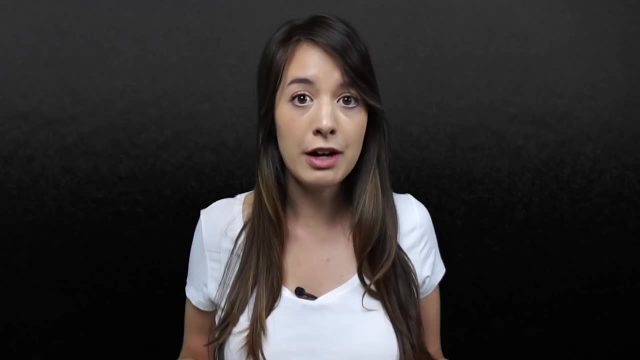 it relies on the laws of physics. It says that you can't know absolutely everything about the state of a quantum particle. It's not because you're not smart enough or your equipment isn't good enough. It's just because nature keeps some things hidden. 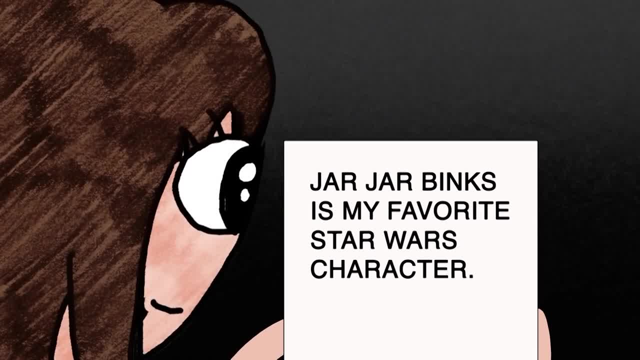 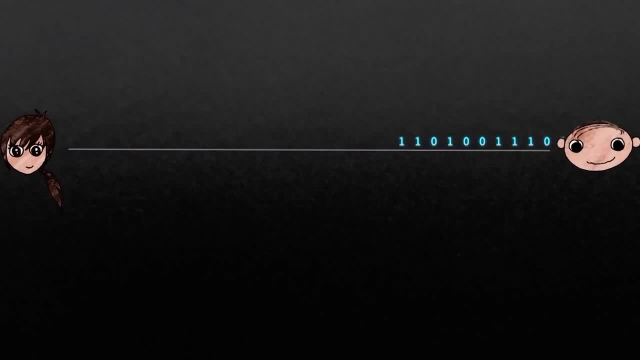 Take this scenario: You want to send Bob a private message. You encrypt the message using a key made up of ones and zeros. You send the key to Bob by a secure line- this could be email or wire- and then mail the message to Bob. 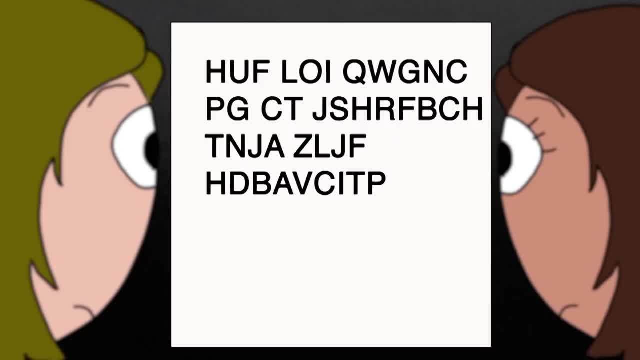 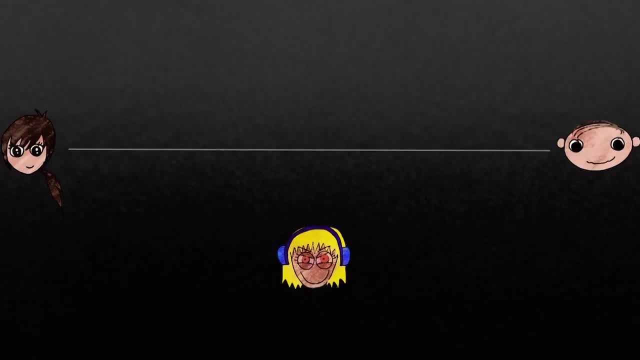 Remember, it doesn't matter if anyone else reads the message. they would be able to understand it. What's important is that no one sees the key, But an eavesdropper, Eve, has tapped into the secure line. Once she has the key, she can read the message and your secret will be publicly known. 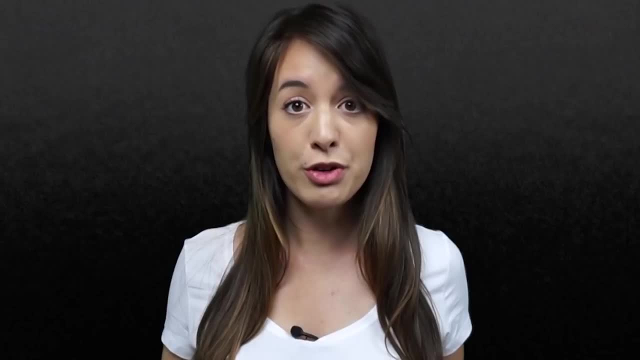 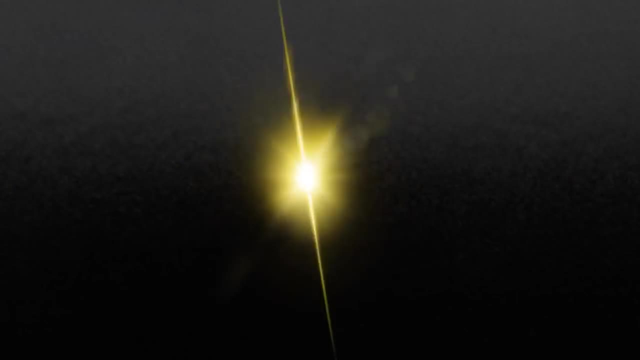 This would never happen if you'd used quantum cryptography. With quantum cryptography, the key is a stream of photons, or light particles. Photons have a property called spin, which can be changed when it passes through a filter. You have four filters. 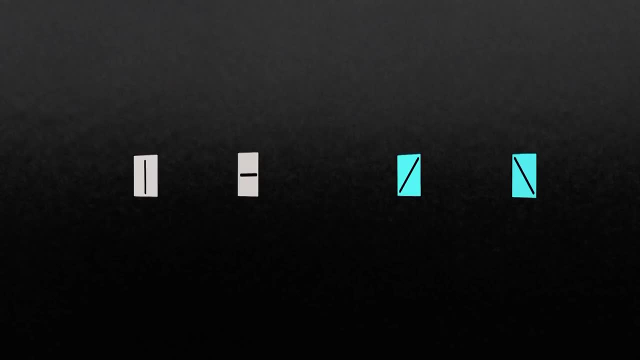 Vertical, horizontal and two-diagonal. We'll lump these into two groups, the diagonal scheme and the rectilinear scheme, To translate photon spin into a key: a photon with vertical or this diagonal spin means one and horizontal or this diagonal spin means zero. 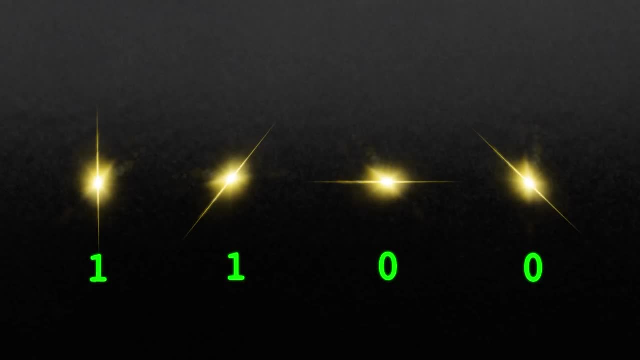 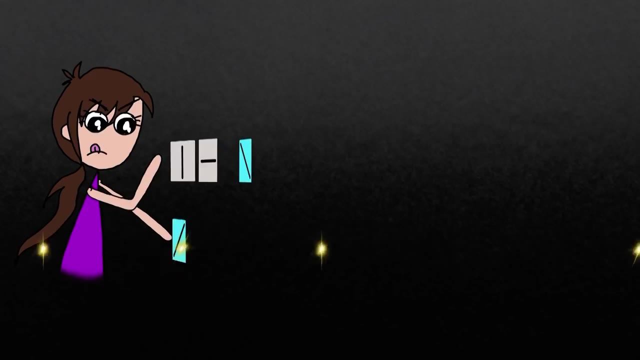 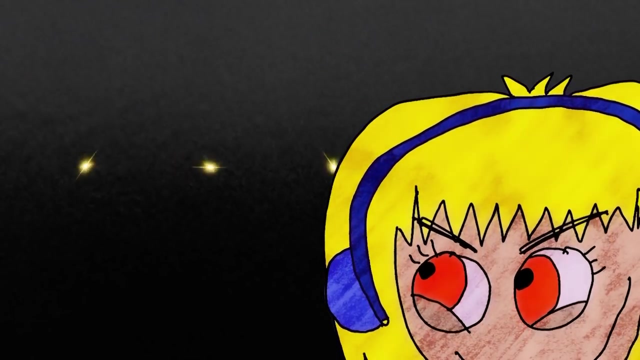 If you wanted to send 1100, you could send this sequence or this one. You start sending Bob photons switching between filters at random. Now here's where the Heisenberg uncertainty principle begins. The only way Eve can measure a photon's spin is by passing it through a filter. 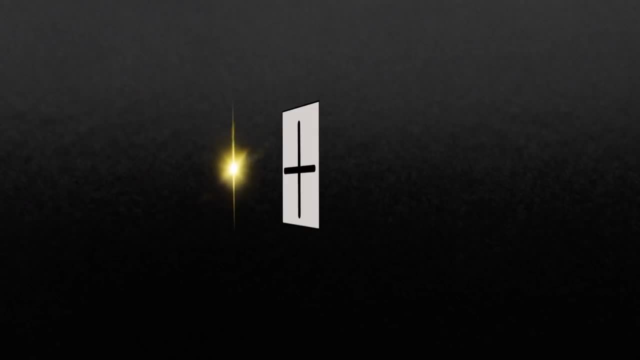 If Eve measures this photon with a rectilinear filter, she'll guess correctly that it has vertical spin and note down a one. But if she uses the diagonal filter, the photon spin will be altered as it passes through. She now incorrectly reads a zero. 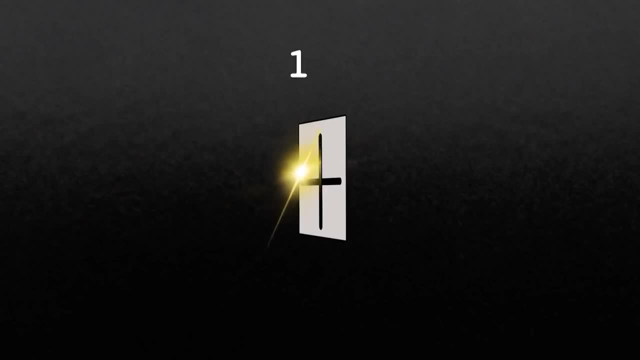 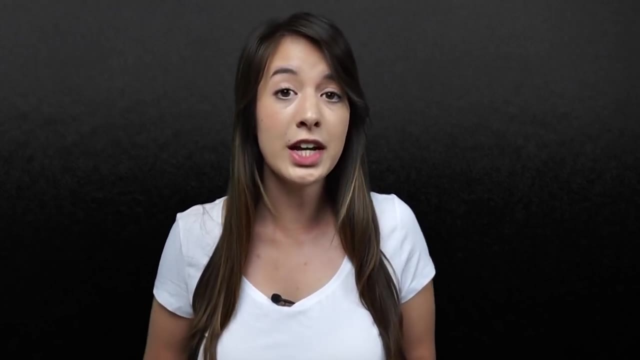 The same will happen if she measures a diagonal photon with the rectilinear filter. Unless Eve knows beforehand which filter to use, she runs a pretty big test. She's taking risk of changing the spin And because you're switching between filters at random,